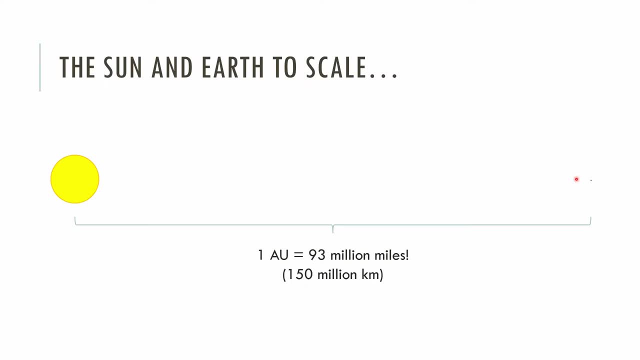 proportionally, we're not getting very much of that, but we're still getting a lot. Remember, energy from the sun accounts for almost all of the energy we use on Earth. ultimately, There's another one to give you another sense of how small the Earth is. 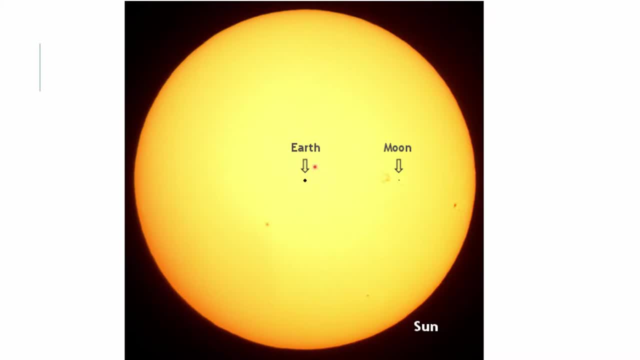 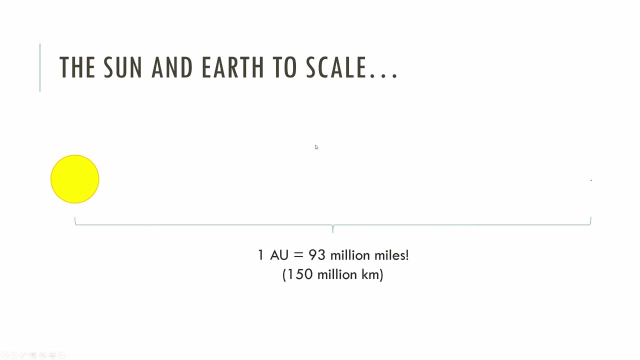 compared to the sun. This is another scale photo, And just for fun, that's the distance between the Earth and the moon and their sizes, the scale as well. So the sun is putting out all this energy, but the Earth, being comparatively very small and very far away, is only going to pick up a small fraction of that energy. 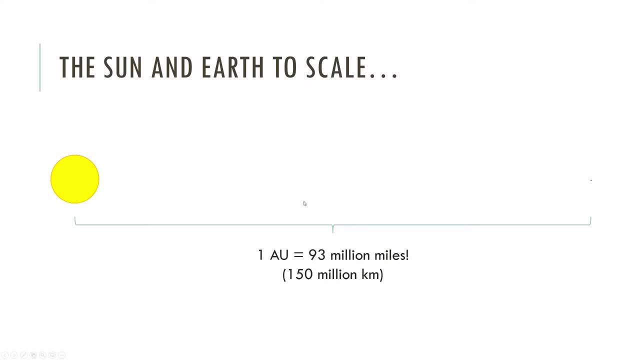 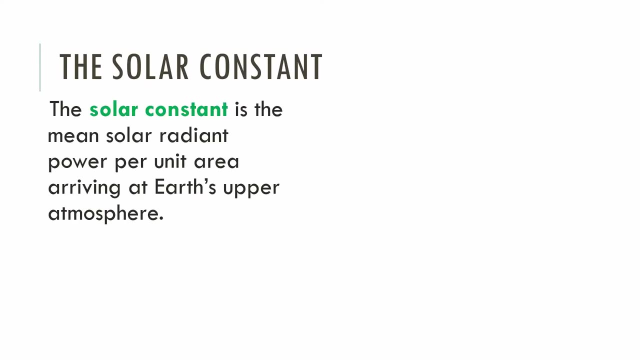 Okay, So the solar constant is the average intensity of the sun's energy at the upper atmosphere of the Earth, And this is the part that's going to get a little interesting. Okay, so, obviously this is definitely not a scale photo, But the idea is we need to measure intensity somewhere. 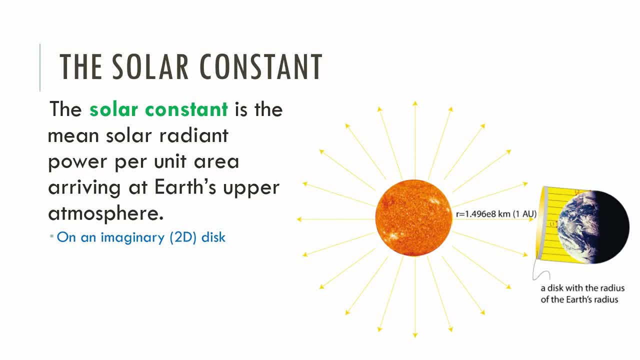 and the atmosphere does all kinds of exciting things, and also the Earth is a sphere, so that's going to get interesting. So for the number for the solar constant, we almost imagine you just go right up into low-orbit space, right where the edge of Earth's atmosphere is. 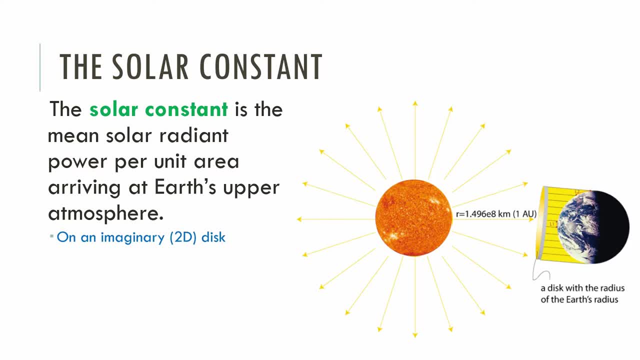 and you put a solar panel And you say: what's the intensity of the sunlight on average? right here, That's the solar constant. You can do this problem. in fact we've done this problem with the inverse square law. 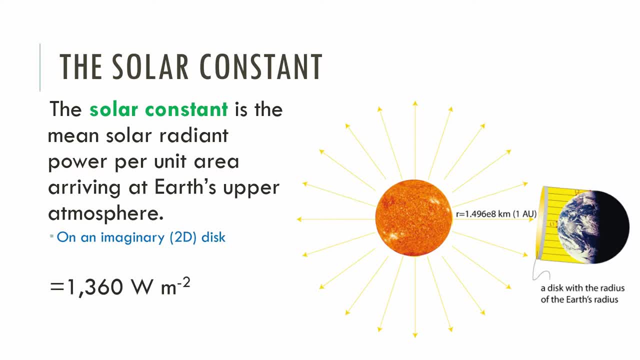 figuring out the power of the sun with the Stefan-Boltzmann law and figuring out, based on how far away we are, what that average intensity would be. It's about 1400,. it's about 1360 watts per square meter. 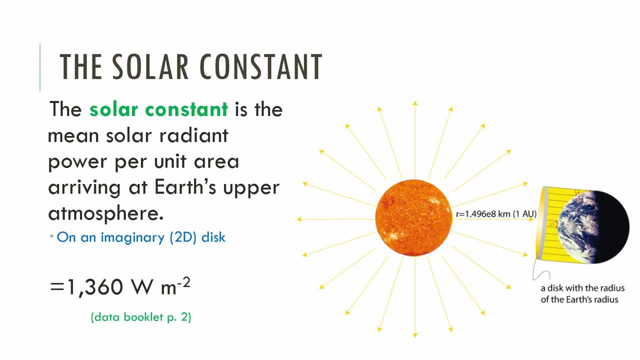 This number is in your data booklet. They give it to you on page two. so you might do problems sometimes with the solar constant. and that's the number Now. it's an average, so of course this kind of fluctuates- The sun does have various amounts of activity, and so on and so on. 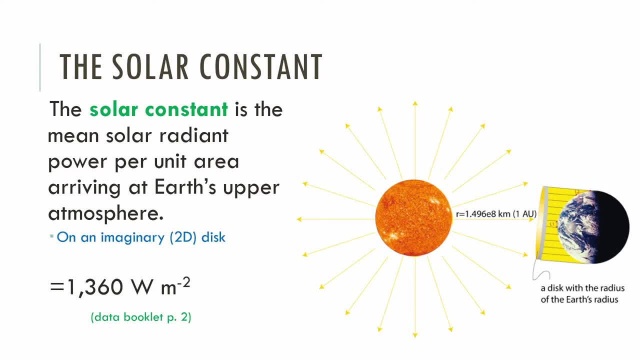 So it's an average, but that's the average power that we get if you were to stick a solar panel right at the edge of the Earth's atmosphere. So that's the solar constant, the average power from the sun at the location of the Earth. 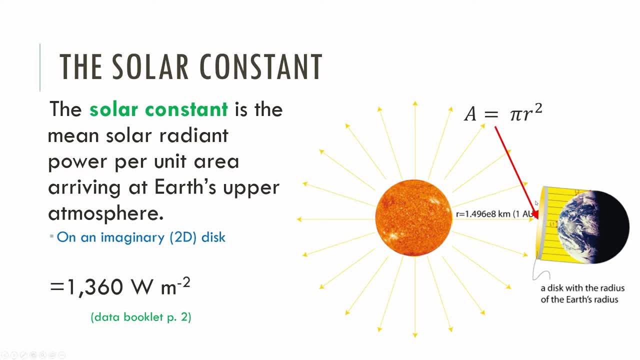 That's how you want to think of it. Where it gets interesting is the Earth is, of course, going to get that energy, but the main kind of wrinkle here is that the Earth is 3D. The Earth is a sphere that rotates. 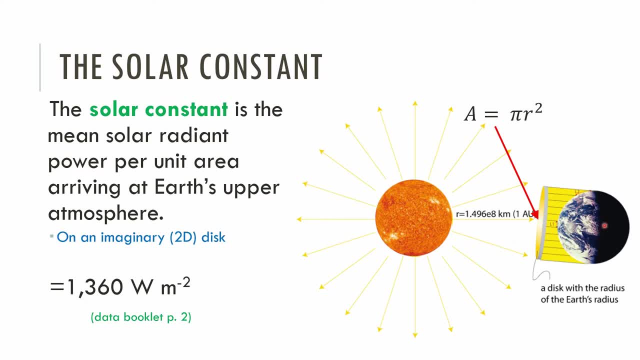 And so there's going to be some parts of the Earth that are getting none of that energy at all at any given time. There's going to be some parts of the Earth that are getting a lot. There are going to be some parts that are getting a medium amount. 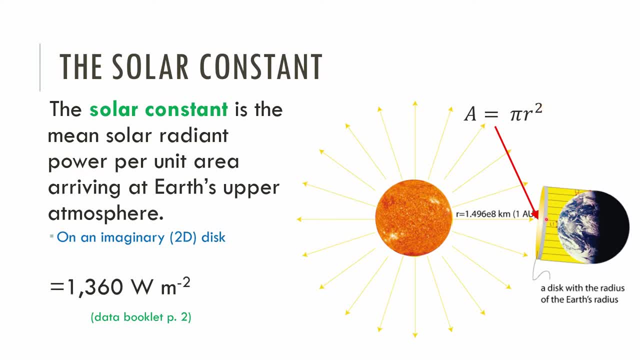 So we need to think about the function of the Earth, We need to think about the fact that this energy is going to spread out over the surface of the whole planet. Okay, so this is a little bit conceptual and sort of just a way to illustrate the idea. 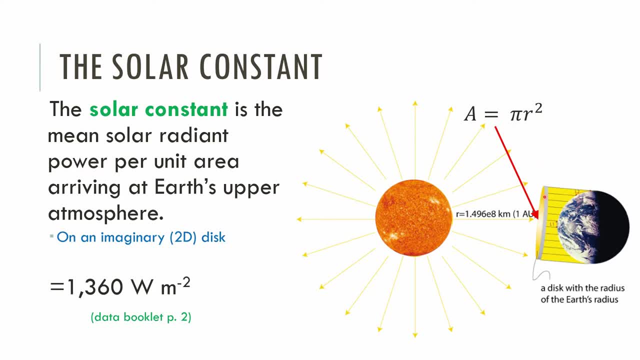 But we could imagine that you take, you make a solar panel as big as the Earth. It's got the same radius as the Earth. So here's this imaginary disk that we're going to talk about. So we, Mr Burns, the world. 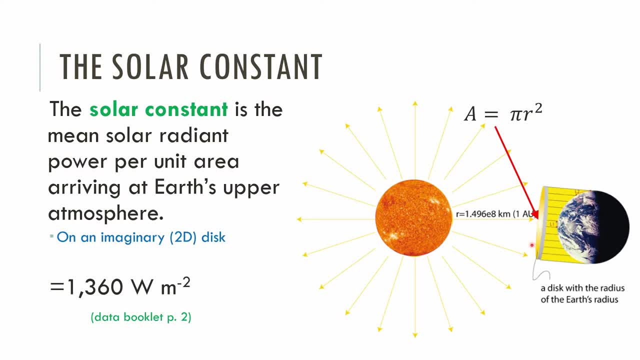 We put a gigantic solar panel That completely covers the Earth to collect all of those 1400 watts per square meter and collect all of the energy here, Instead of letting that energy spread out over the surface of the Earth. Well, if you do that, the area of this disk would be the area of a circle pi r squared. 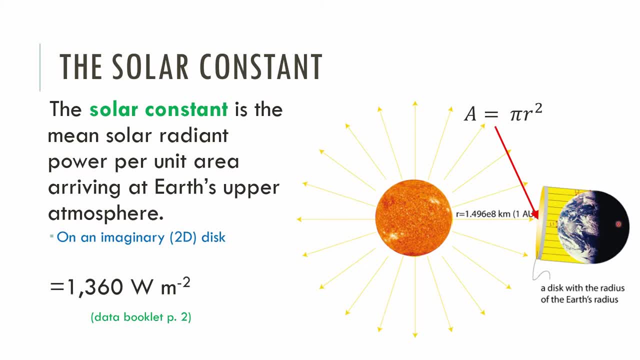 But that's not what we have. What we have is that energy gets smeared out over the entire surface of the Earth during the course of a day and a year and so on, And the The area that it really gets spread out over is the surface area of a sphere. 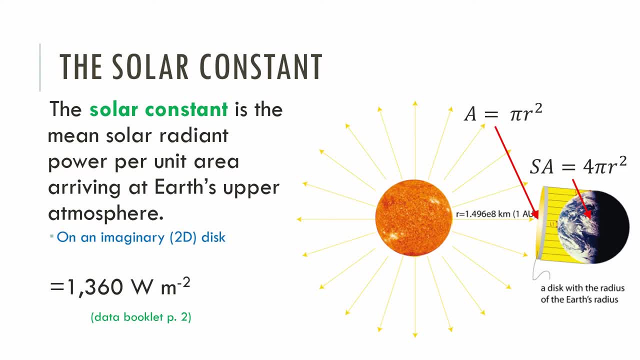 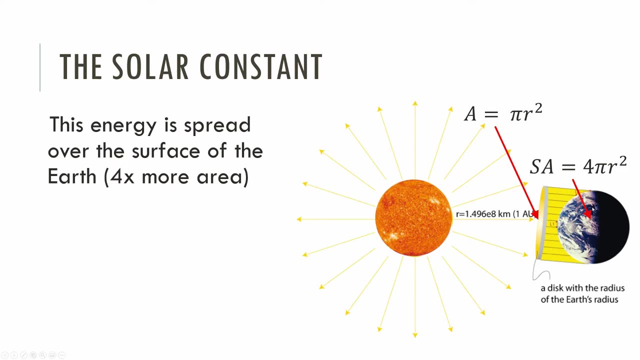 which is 4 pi r squared Four times more area. So we get this 1400 watts per square meter on this kind of imaginary disk. But what we really care about is how much we're going to get here. Well, the area is four times bigger, so we're going to get four times less. 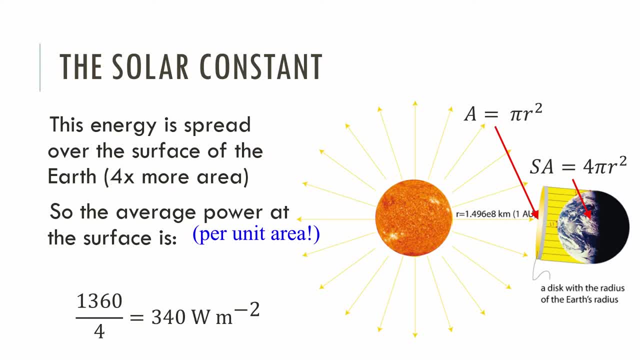 So what we really have practically to work with in terms of being on the Surface of the planet On average, considering the fact that the planet rotates and is not always in direct sunlight- On average you're going to get 340.. You divide the solar constant by four. 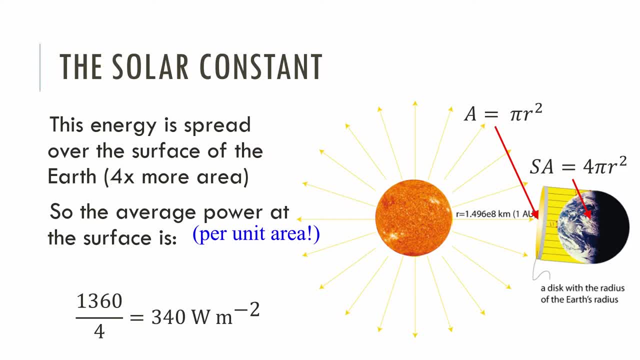 The IB will ask you to do this and they'll ask you to explain why. And the reason is: The solar constant involves the average intensity in the upper atmosphere on an imaginary disk And in reality that power spreads out over the surface area of. 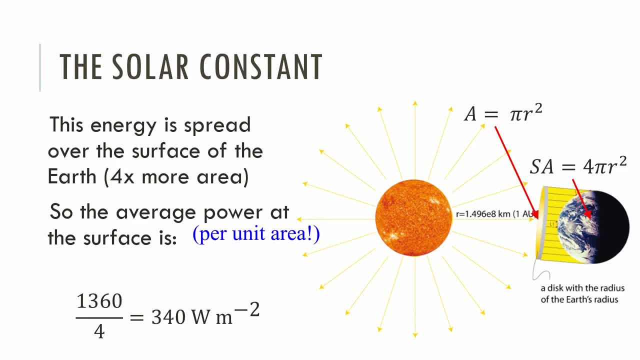 The planet, which is a sphere, And they want you to say something like. the surface area of a sphere is four times more than the surface area of a disk, So therefore the power per area is four times lower. So the average intensity at the surface of the planet is going to be about 340.. 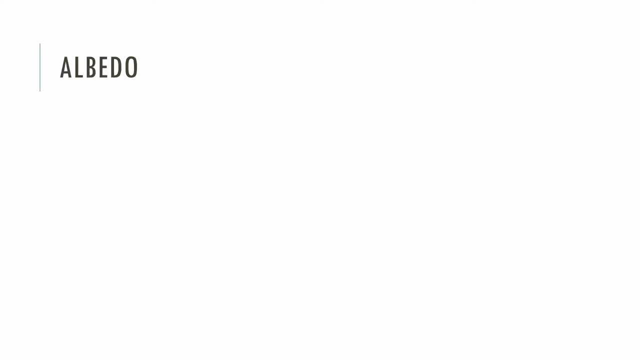 The solar constant divided by four. One other concept to talk about. another number related to the sun's light at the earth is albedo. This is a percentage. This is basically going to look at how much of the sun's energy gets reflected away by the planet. 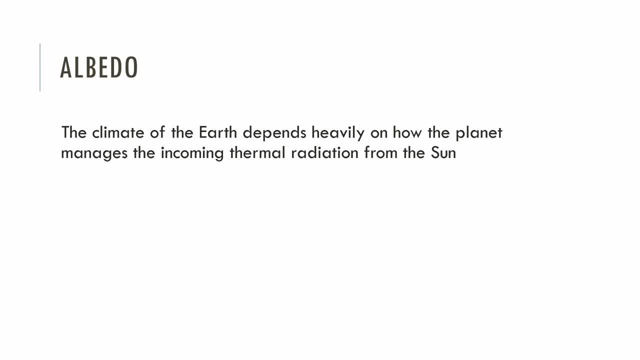 And that's what albedo is. This is going to be really important in terms of talking about the climate of the planet, which we'll get into, But basically it's how we manage this radiation, how we form some kind of equilibrium. 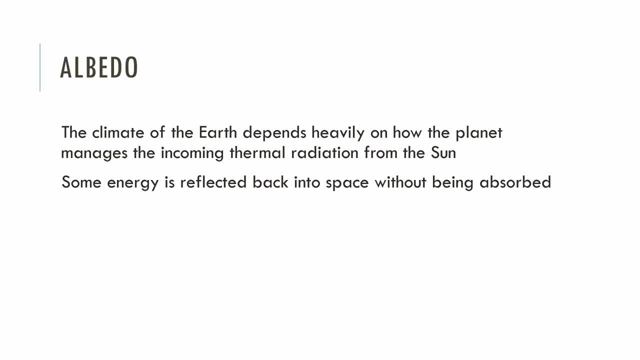 So the amount that we reflect away is going to be important. There's a: the earth is not a perfect black body. It's not, in fact, nearly as good a black body as the sun, even though We'll sometimes model it that way. 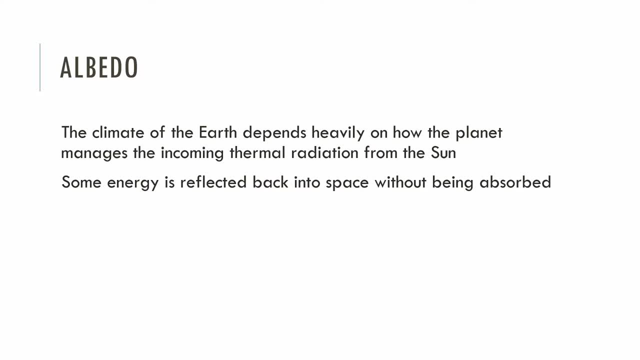 But the earth does reflect away a good amount of the energy coming from the sun's light, And albedo will measure the amount of energy that a body reflects back into space. We'll say scatters to scatters is essentially a synonym for reflects. 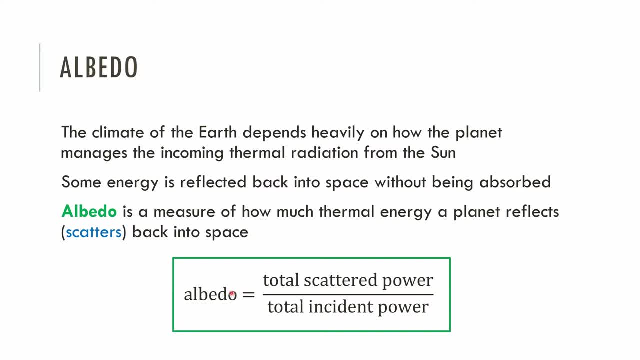 So here's the equation in your data booklet: albedo. It's just a word equation. Albedo is the total scattered power divided by total incident power, In other words, how much It's reflected by divided by how much comes in. So we're always going to end up with a decimal, with a percentage. 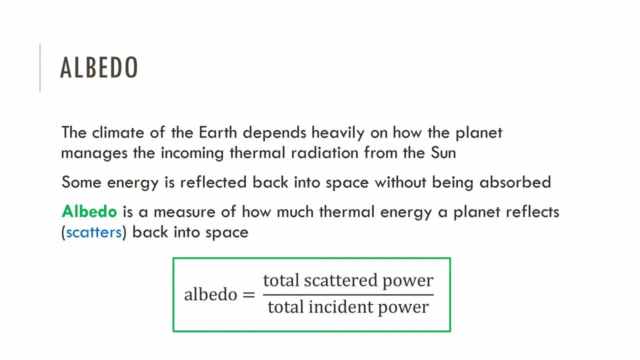 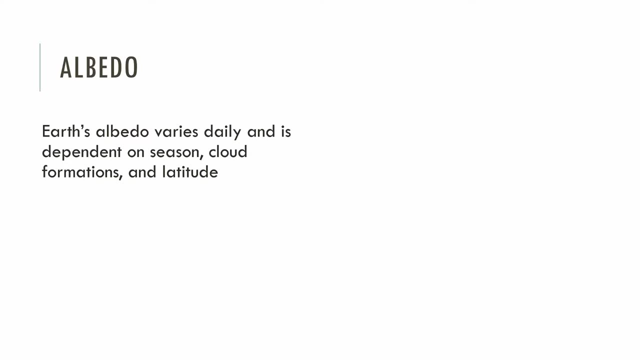 So it's a percentage of. at the end of the day, Really, all you need to think about here is that albedo measures what percentage of the light from the sun or the nearby star gets reflected away. This is another example where we're really talking about an average. 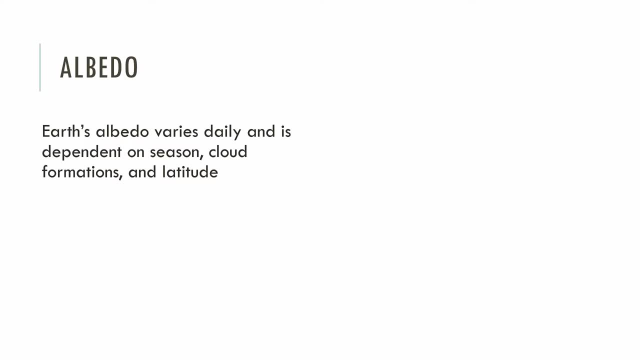 It changes a whole lot depending on where you are on the planet, what the season is, The tilt of the earth at what the cloud formations are doing on that particular day. It's very different based on latitude. So we're what we're really going to look at, similar to the solar concept. 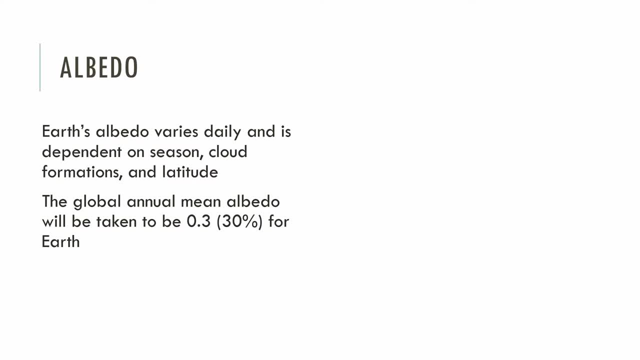 We're looking at an average, the global annual mean albedo. So over the course of a year, considering the whole planet as a big thing, the average is about 30%. about 30% of the sun's light gets reflected back into space by the earth. 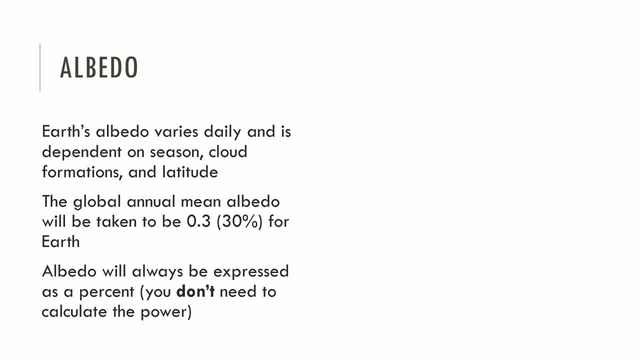 It'll always be a percentage, even though Equation kind of says power over power. You don't really ever need to calculate those power numbers. You're going to get stuff like this. There've been lots of IB questions in the past that look like this: 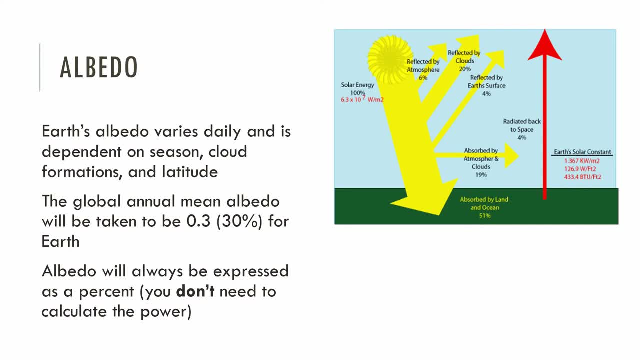 They give you sort of a diagram and show all these different arrows and they show some stuff getting absorbed and some getting reflected. So here we have a hundred percent of the input energy. This is just the energy from the sun's. what's a hundred percent the input? 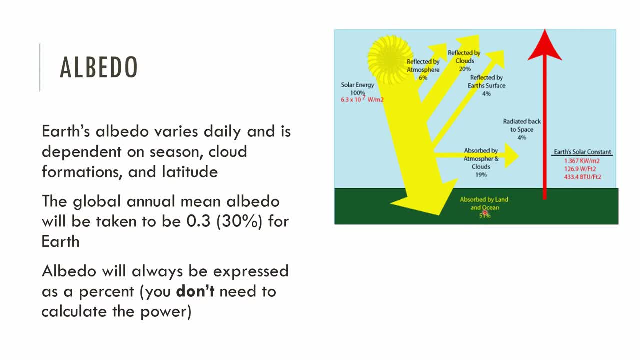 And in this example, you know, 51% is absorbed by the land and ocean, 19% is absorbed by atmosphere and clouds. Some of it gets radiated back into space, because the earth itself is a black body, but they also show. maybe 6% of it gets reflected by the atmosphere, 20% reflected by clouds. 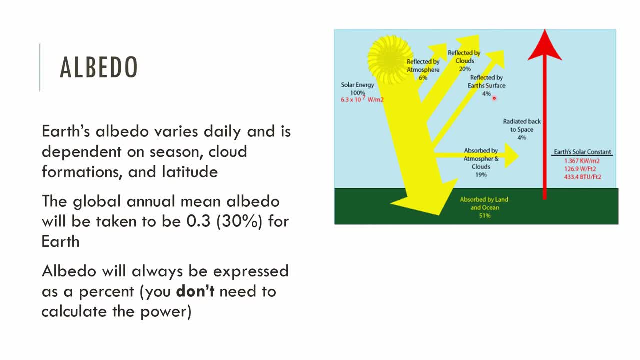 4% reflected by the surface, And all you do for a problem like this is you just add up all the reflected percentages and that's your albedo. So 6% gets reflected by atmosphere: 20 clouds, four surface. add them up: 30%, 0.3 or 30% is the albedo. 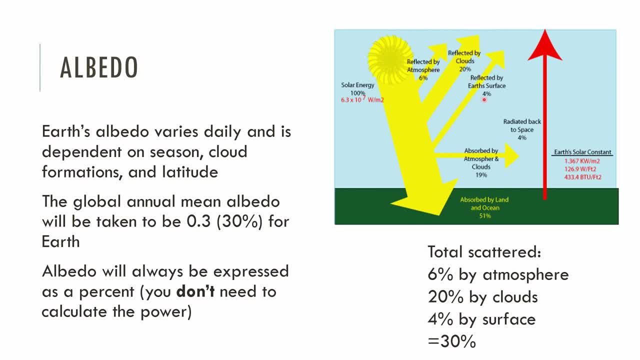 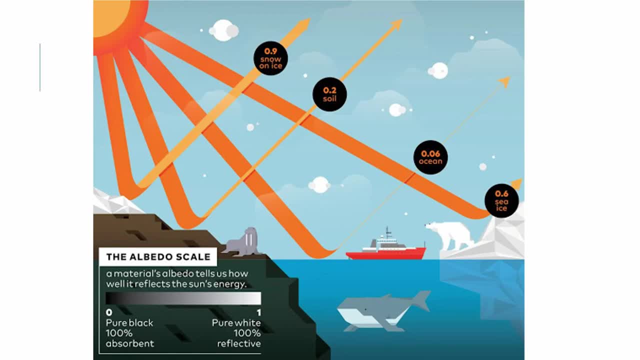 In this kind of problem. So a lot of times the calculating albedo is as easy as that. You just add up all the stuff that gets reflected, Okay, So, uh, just to give you a sense, because we'll we'll get into this a little bit.